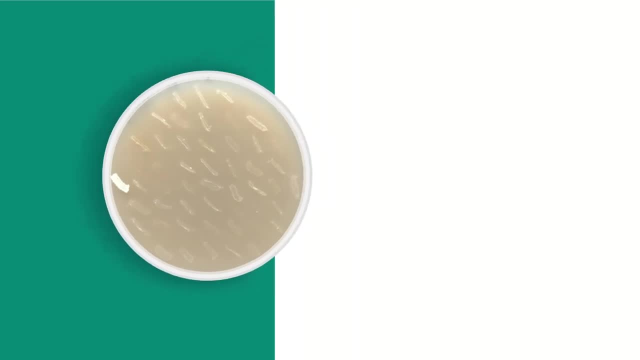 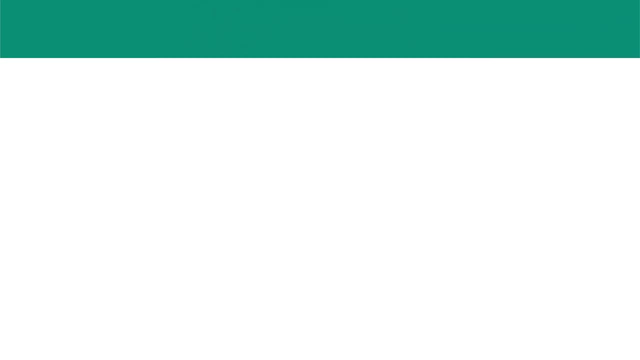 rather unimpressive populations growing in the streak marks. You can improve soil health by adding phycoterra and increasing the total abundance and diversity of the system. The next piece is the counterpart, soil quality. So soil quality is a little bit older in usage. 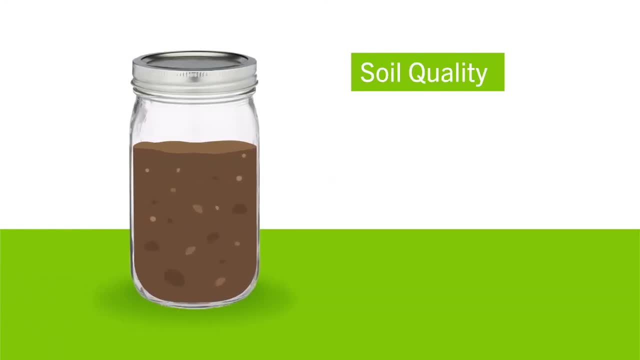 and it also has a much broader application. Soil quality refers to how well the soil functions physically, chemically and biologically and how well that soil does its job. On an agro ecosystem like a farm, the soil's job is crop production. But if you think 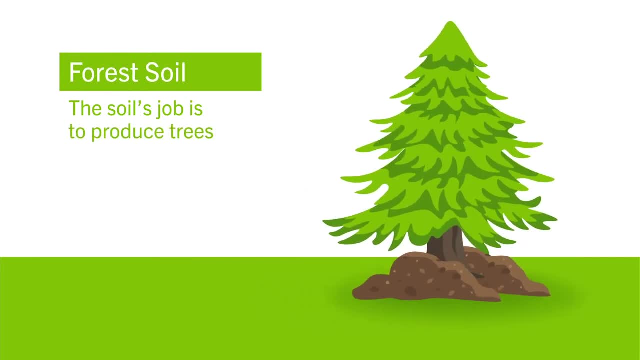 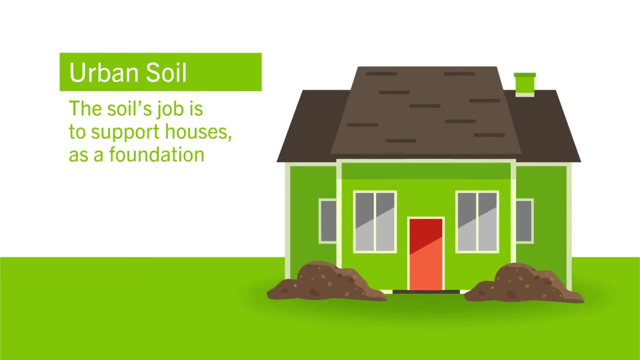 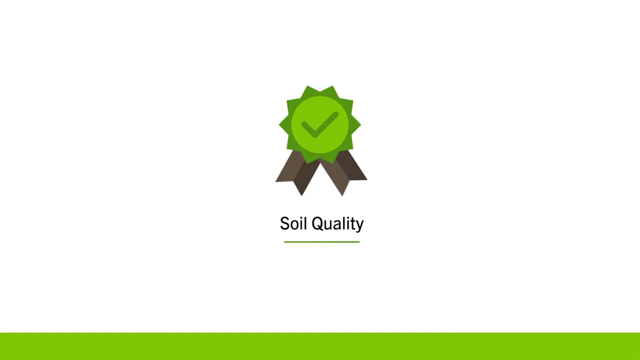 of the job. in a forest soil it's much different. That's to produce trees. If you think of an urban soil, that soil's job might be to support houses and as a foundation So that job can change. and that's a measurement of soil quality. But in this example we refer to soil quality in the 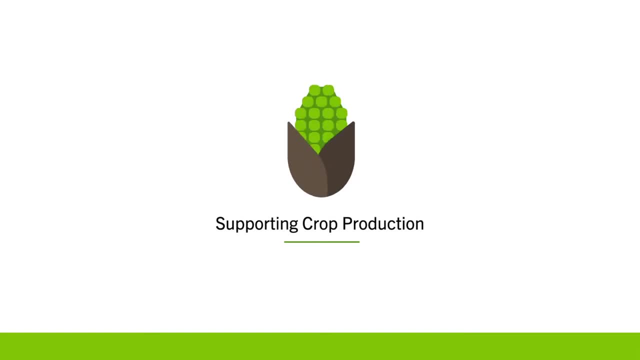 farm sense supporting crop production. So here's a way to think about soil quality and its relationship to the farm system. Soil quality can be linked to changes in the soil structure. Here is the untreated control across many different textures: Silty, clay, sand, loam. 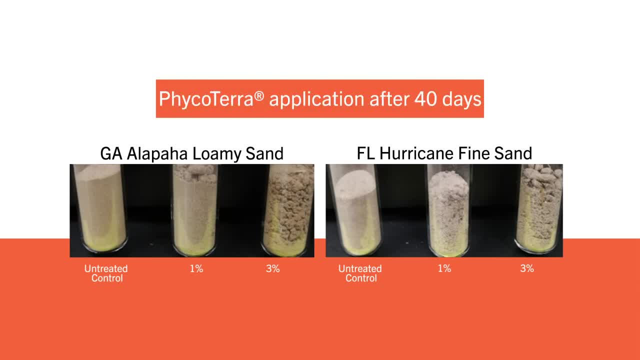 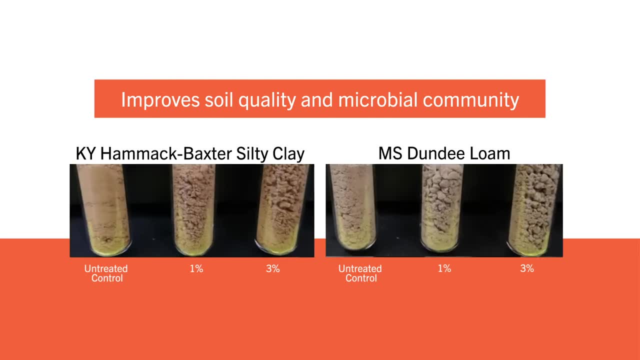 fine sands all over the map. here We add the phycoterra and we can improve soil quality from the control by adding that microbial food source, improving the microbial community, which then helps stitch your soil back together. You can increase the agglomeration or aggregation of the soil. and it's that same agglomeration that makes the soil better. You can increase the agglomeration or aggregation of the soil, and it's that same agglomeration that makes the soil better. You can increase the agglomeration or aggregation of the soil, and it's that same aggregation response. 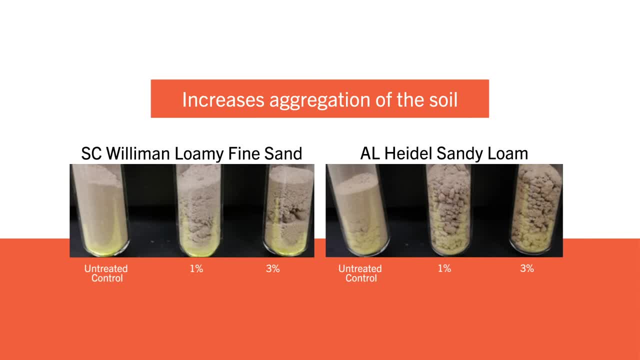 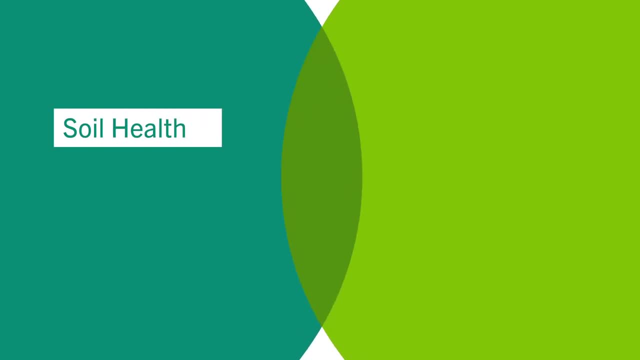 that's shown on the far right of each of these pictures. That's an improvement in soil quality. Now I mentioned the soil-microbe connection, that's soil health. Soil health and soil quality go hand in hand- two different terms, but it is important to keep in mind that they're more like a Venn diagram. 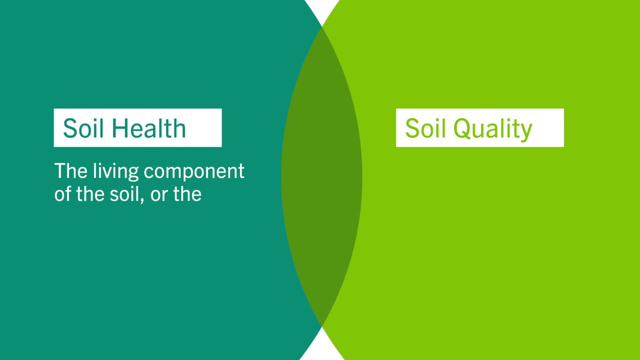 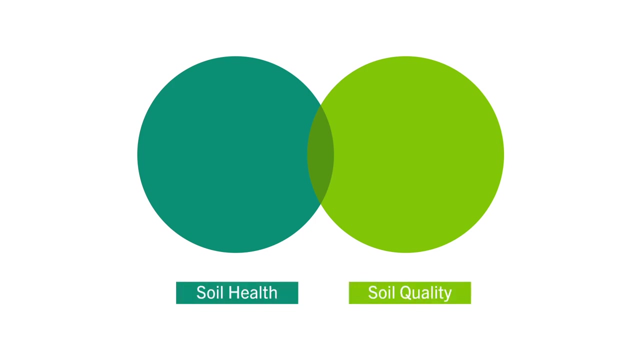 One focuses on the living component of soil, the soil health and biological integrity, and the other focuses on the more physical aspects, or soil quality and how well that soil does its job. Soil health and soil quality are two different concepts. There are some subtleties to how they're.